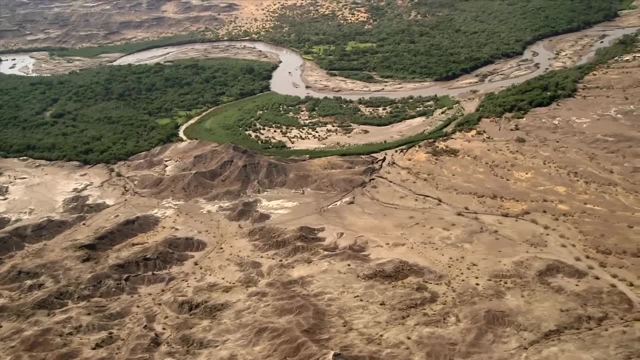 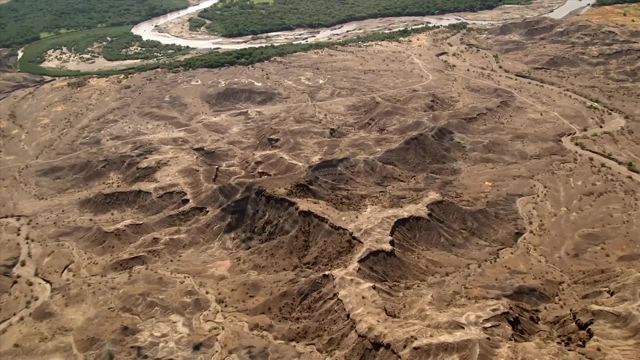 Look at those rocks. It's boom, boom, boom, boom, boom, Just totally stretched out. As a paleontologist, that is what I dream about. You guys see the volcano. You see the volcanic ash cropping out. That's 3.4 million years old. That is incredible. 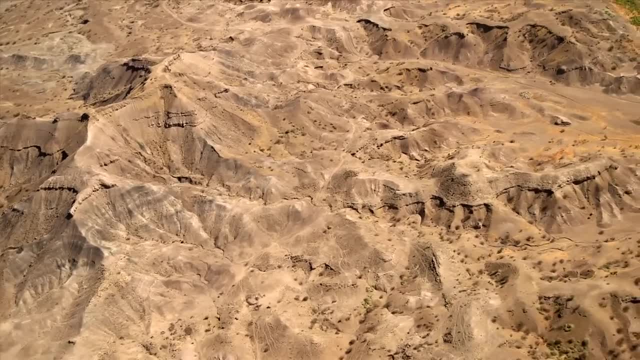 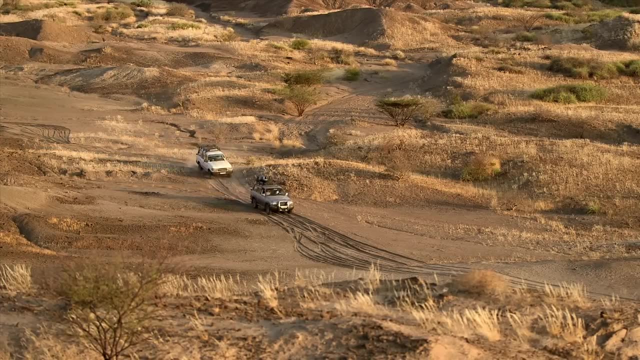 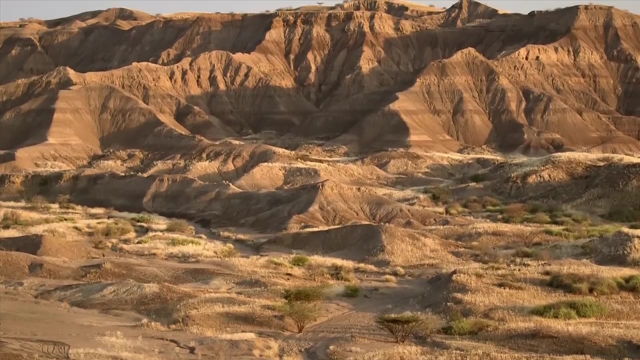 One of our unique characteristics is walking on two legs. The question is: what did our ancient two-legged ancestors look like? A fossil found here in the Afar region of Ethiopia gives us a pretty good idea. Don's taking me to see where he found a 3.2 million year old hominid known as Lucy. 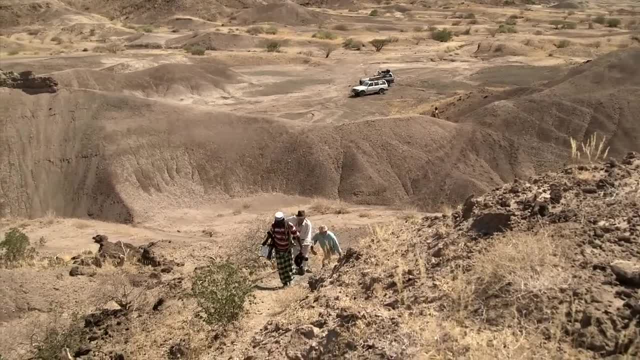 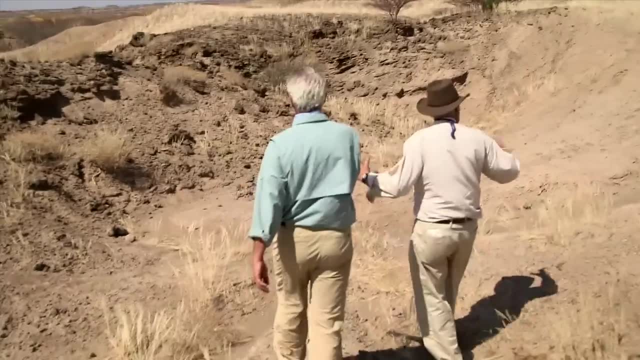 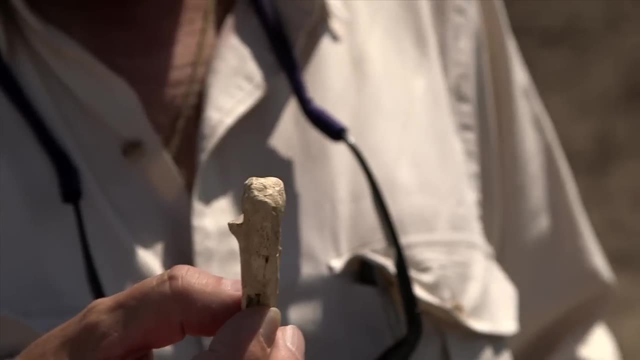 It was a Sunday morning back in 1974. So I came up here, looked at this, had no idea what was waiting. It was right in this area, right here. What I saw was a fragment of bone and I looked at it and almost instantaneously said that's a hominid. 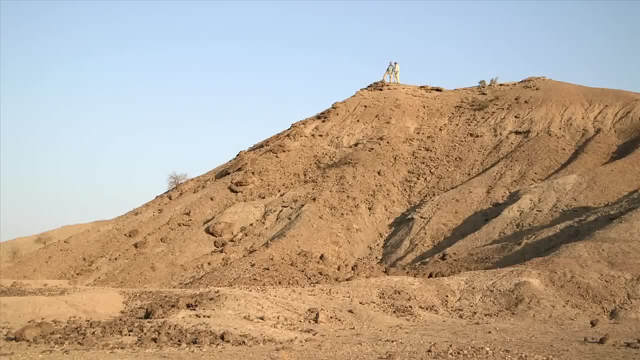 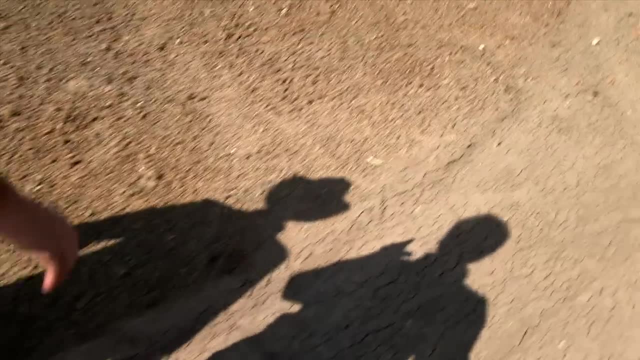 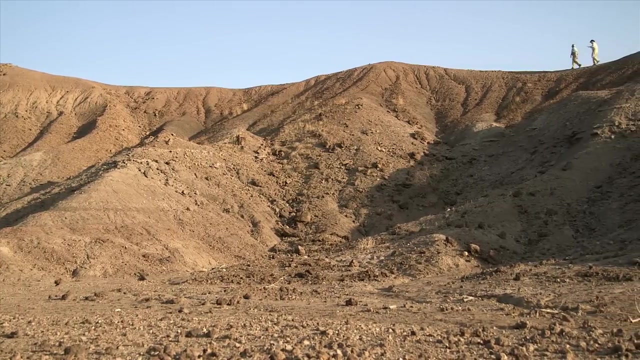 Wow. Once we broke that 3 million year barrier, it was a whole new picture of what our earliest ancestors looked like, One of the most exciting moments of my life, My entire career. Lucy made headlines around the world because, although she looked a lot like an ape, she walked on two legs. 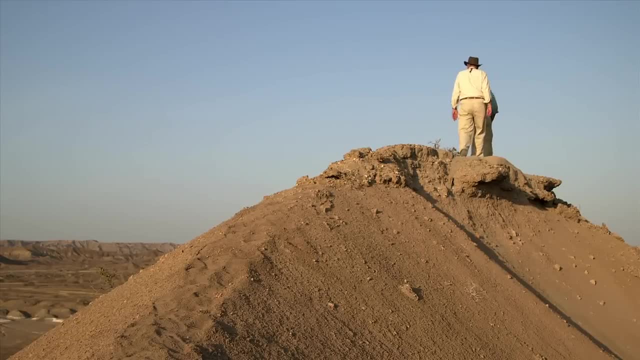 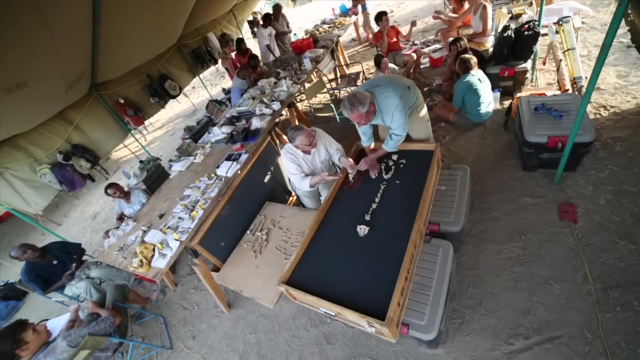 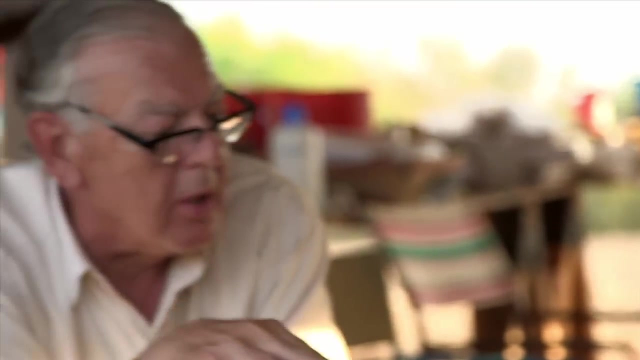 She was a biped and, at that stage, the most ancient anyone had ever found. Her bones are some of the best evidence we have for what early bipeds looked like. Now, of course, if this were all articulated properly- you know the vertebrae on top of it, you know you'd be a bit of a pain in the ass. 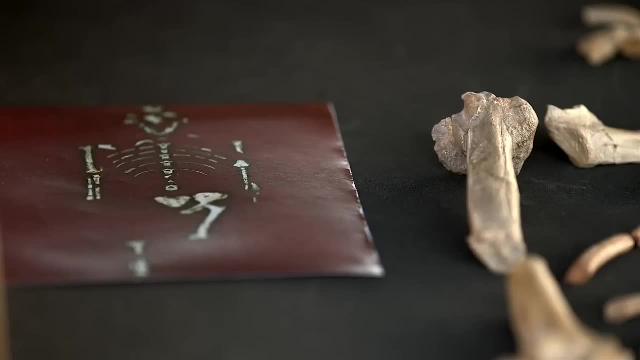 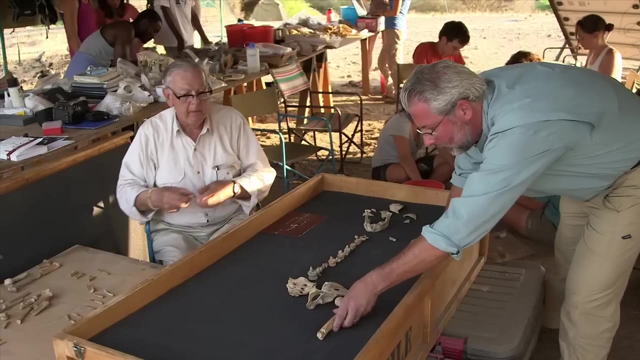 You'd see, She'd be about three and a half feet tall. You don't see that? Yeah, you don't get that. Here's the femur, That's the left Top end of the thigh bone, And this one also. I mean, when you put it all together now you have. you know, this is telling bipedal, this is giving a hint of bipedal. 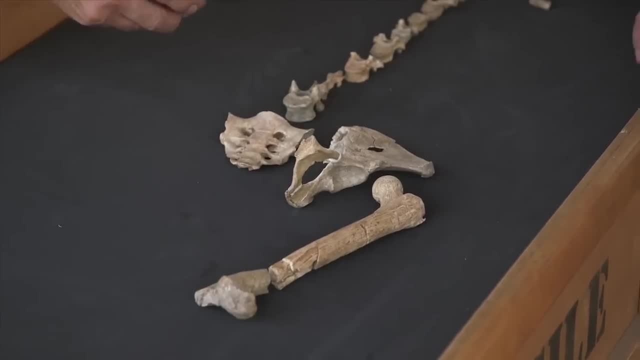 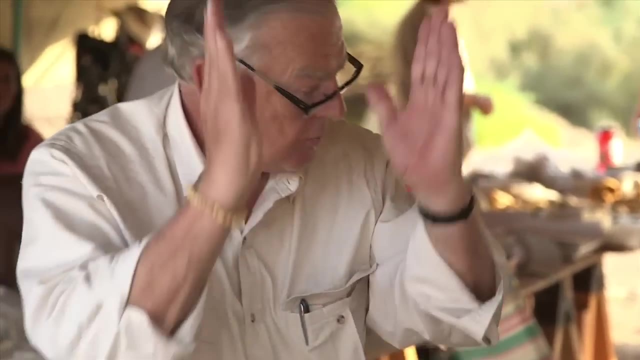 This certainly tells it was bipedal. That can't in like that, which is very characteristic. Our knees are close together and they come up to the side. The chimps come straight up, So that's another very important aspect: Having the upper.